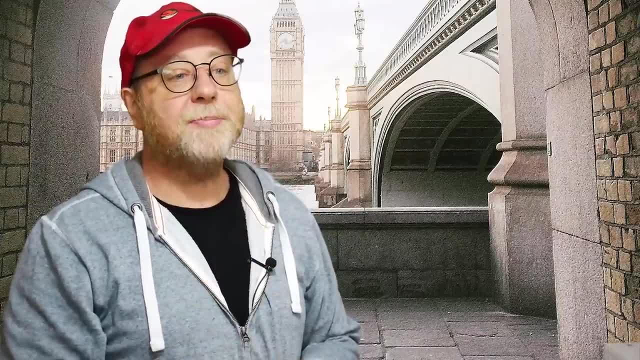 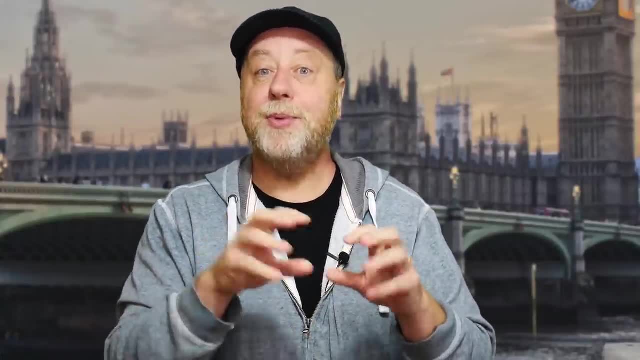 past 12 and 30 seconds. Hey, Gary, Gary says it's four minutes past 12 and 30 seconds. Okay, thanks. Now that's how we might ask what is the time. but the question is: how does a computer ask what is the time? Well, if you want to find out more, please let me explain. 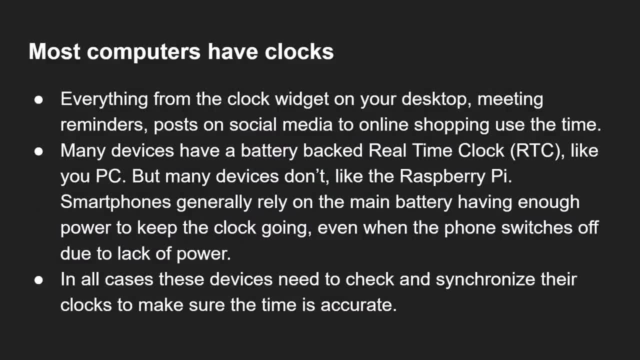 Okay. so most computers have clocks and everything from the clock widget on your desktop, meeting reminders, posts on social media, online shopping- they all use the time. Now many devices have a battery-backed real-time clock RTC, like your PC, for example, but some devices don't. 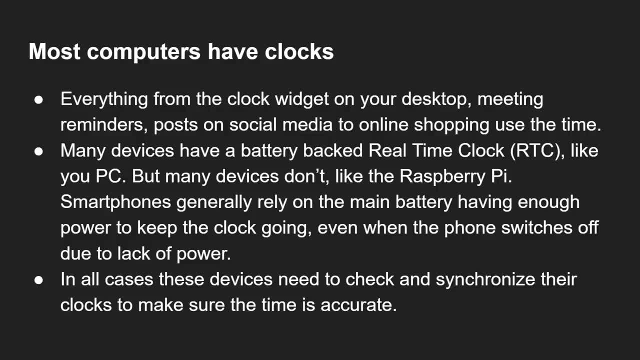 For example, the Raspberry Pi does not come with a battery-backed real-time clock. Smartphones rely, of course, on the main battery to have enough power and even when you're phone shuts down, there's often still enough power to keep the clock going. But in all cases, all of 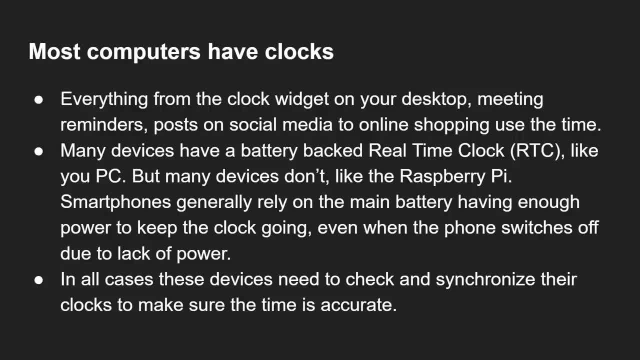 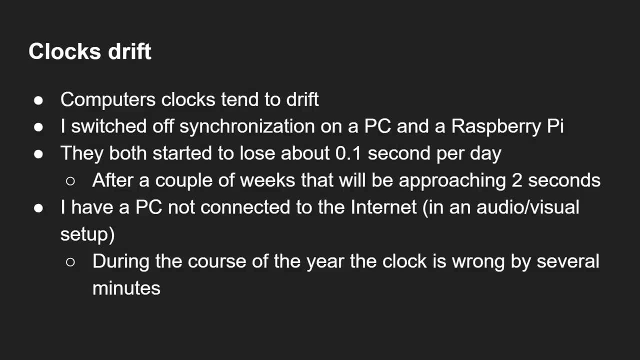 these devices need to check they have the correct time and synchronize it to make sure it is accurate. Now computer clocks tend to drift because they're not really a very expensive part in the whole kind of sum of everything. So, for example, I switched off synchronization. 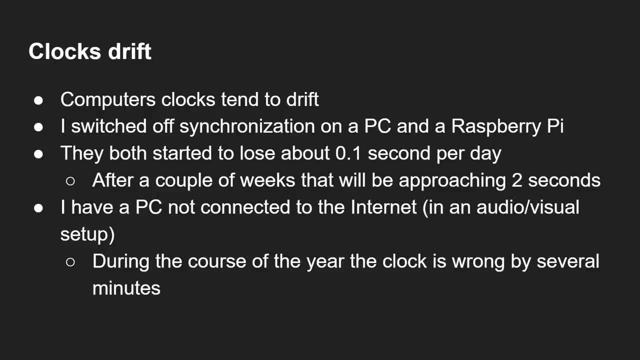 on a desktop PC and on a Raspberry Pi and they both started to lose about 0.1 seconds per day. So I switched off the RTC on a desktop PC and on a Raspberry Pi and they both started to lose about 0.1 seconds per day. So, for example, I switched off synchronization on a desktop PC and on a Raspberry Pi and they both started to lose about 0.1 seconds per day. So, for example, I switched off synchronization on a desktop PC and on a Raspberry Pi and they both started to lose about 0.1 seconds per day. 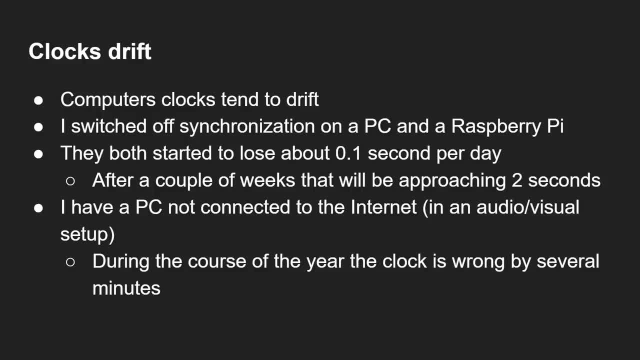 Which means after a couple of weeks they'll be about 2 seconds out. Now I have a PC that I use that's not connected to the internet at all. It's an audio visual setup that I have to use and during the course of the year that clock can be wrong by. 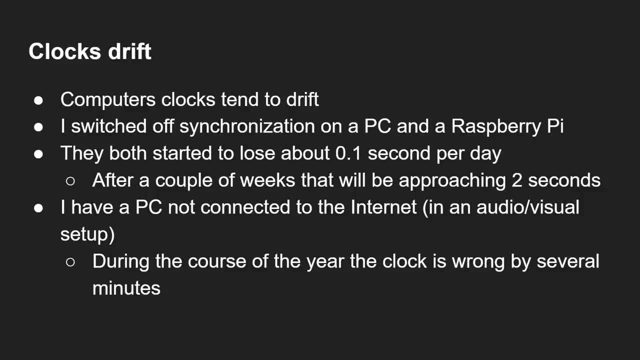 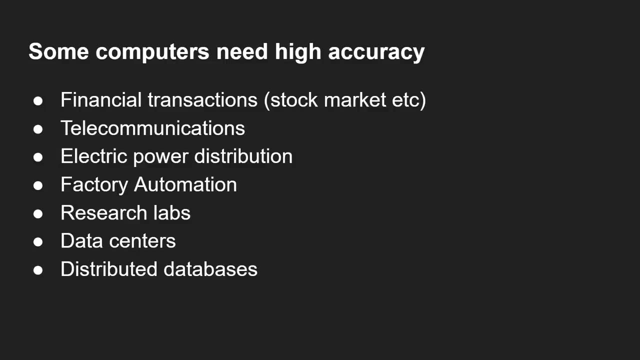 several minutes. So it's very important that computers synchronize their time to actually get the correct date and time for all the things that we do, The simple things we do, like emails and buying things online. But there are some computers that need very, very high computer accuracy for time, For example, financial transactions in a stock market. 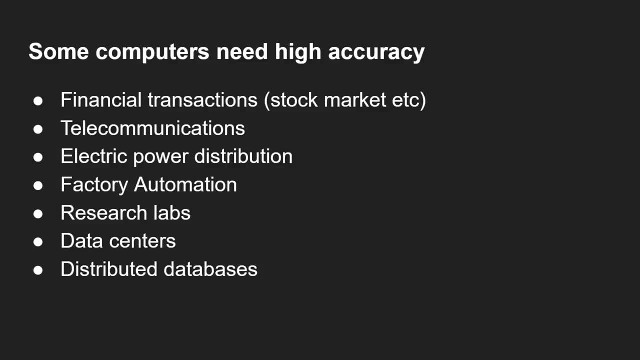 Fractions of a second. Who got that buy order or that seller order in first becomes important. The same with telecommunications, power distribution, factory automation. All of these areas need sub one. second, They need very good accuracy for the clocks Research labs. 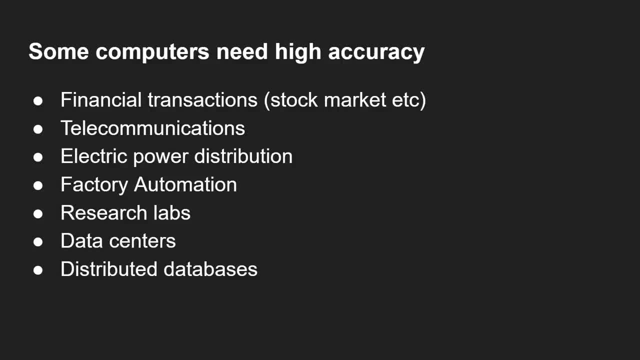 If you're doing particle physics research, then you need even greater definitions. accuracy of time: Data centers need accurate time. Distributed databases particularly need accurate time. So it's not only for the stuff that we do Simple things like social media or buying. you know a new. 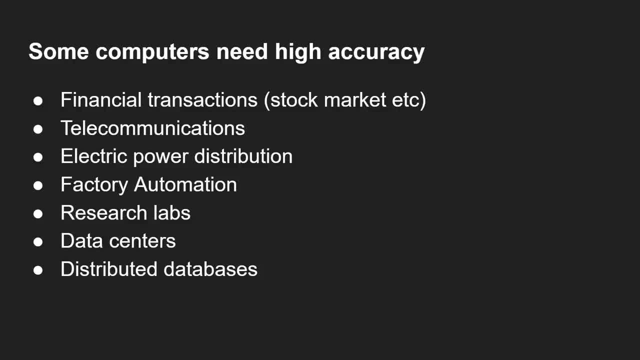 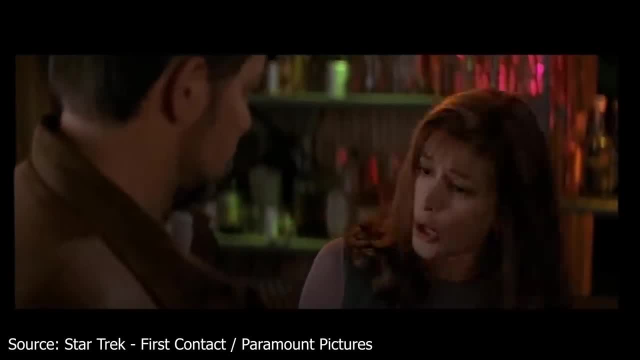 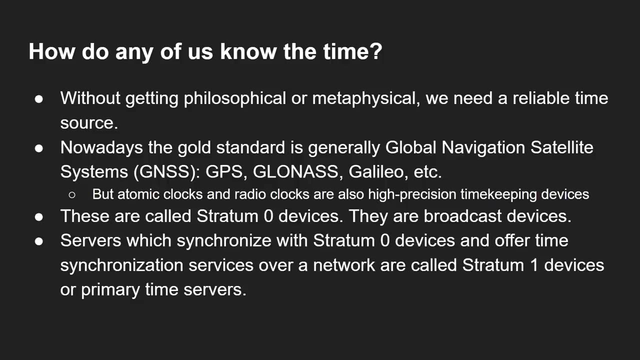 packet of tissues online. There are some areas where really really high accuracy is important for the jobs that the people are doing. This is no time to argue about time. We don't have the time Now. how do any of us know what is the time Now without getting philosophical? 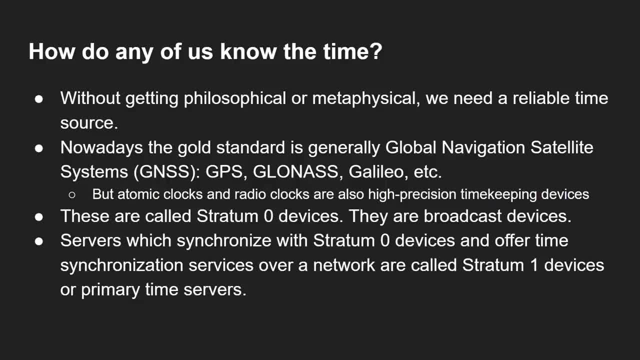 Or metaphysical. We need a reliable time source. Now, that's not going to be the watch on your wrist, It's not going to be the kind of the clock on your kitchen wall. Okay, we need a gold standard. At the moment, that's generally global navigation, satellite systems, GNSS. 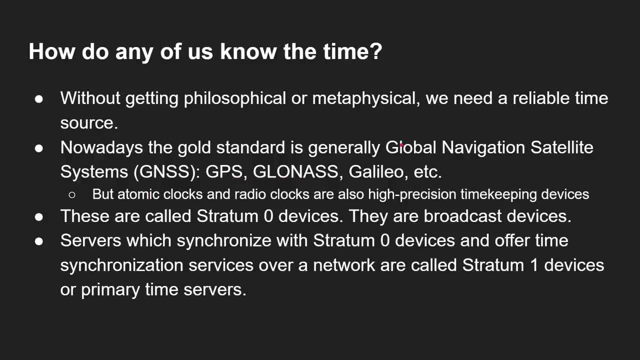 Which includes GPS, GLONASS, Galileo, and there are. there are several others. Of course, there are also atomic clocks and radio clocks and these also offer high precision time keeping- Now, these level of, you know, atomic clock kind of things. Of course, GPS satellites. 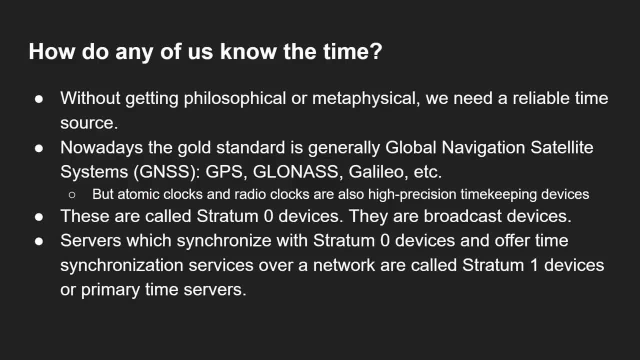 and they've got atomic clocks in them. Atomic clocks are generally called stratum zero devices and they broadcast the time. Of course, that's the whole way that global navigation satellites work: They broadcast the time and you can work out your- your position based on the time. Now servers somewhere will synchronize with a stratum zero. 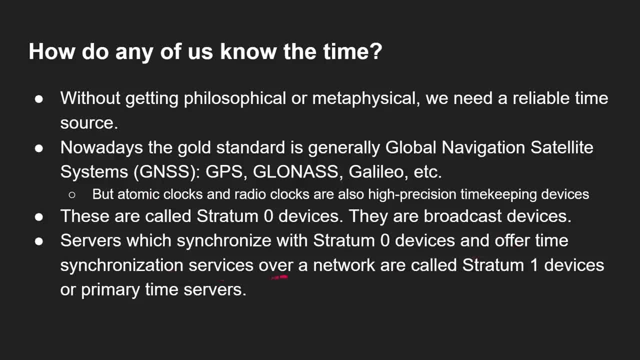 device and they will offer synchronization services over a network, And they're called stratum one devices or primary time servers. So there are lots and lots of these primary time servers dotted around all around the world, And then you can actually have further servers that are further connected to them. So what you actually get then is this layer approach, stratum. 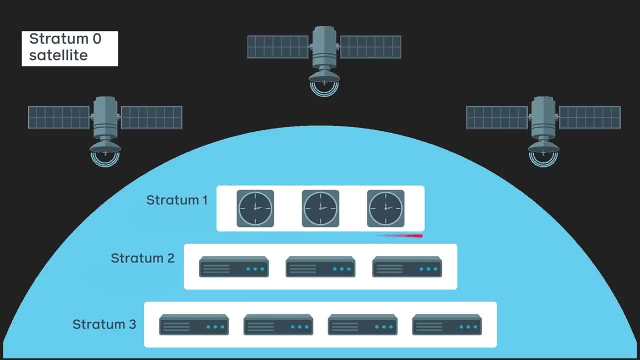 So stratum zero is the satellites, Stratum one maybe these primary time servers. who's kind of connected up to all these? Maybe connect up to a radio clock, to an atomic clock and they really know the time, And then you get these servers that are connected to them directly. 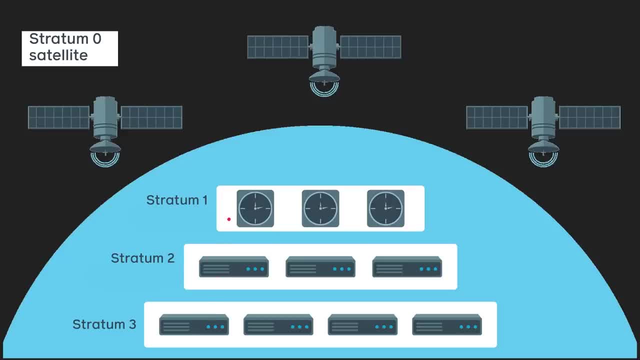 And then other servers would connect to them And you can actually get up to 15 layers of stratum. Once you get to the 15th layer you you're not allowed to take the time from the 15th layer one, because that is the bottom layer, But from 14 upwards. But generally we get one, two. 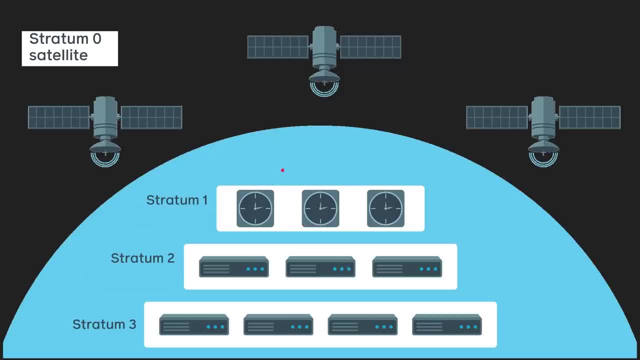 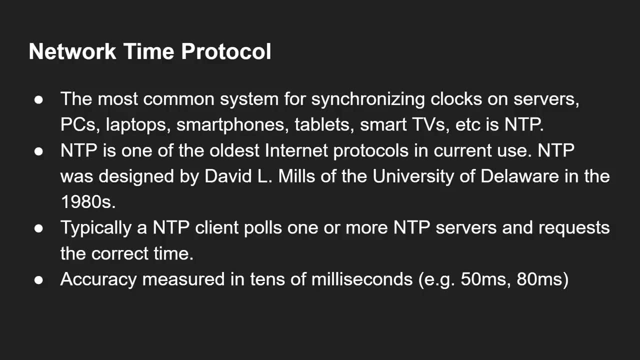 three, maybe four kind of knocking about on the internet. Now the most common system for synchronizing clocks on servers- PCs, laptops, smartphones, tablets, smart TVs, etc. is NTP, The network time protocol. Now, NTP is one of the oldest internet protocols that's currently being used. It. 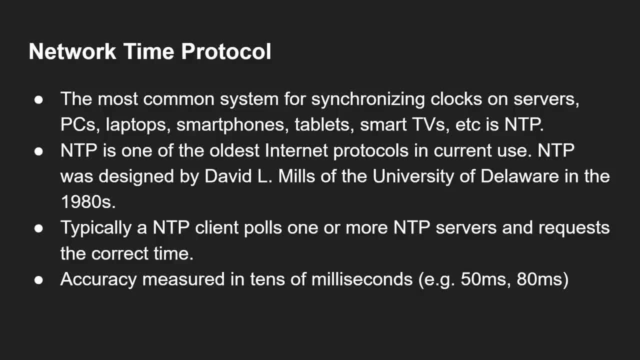 was developed by David Mills of the University of Delaware in the 1980s. Now, typically, an NTP client polls one or more NTP servers and requests the current time. the correct time And accuracy is normally measured in tens of milliseconds, So you know that the clock on your PC is accurate. 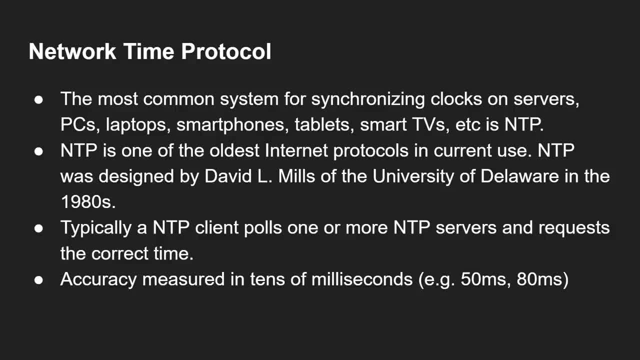 within 50 milliseconds, 80 milliseconds And, of course, if you don't have a grasp of milliseconds, microseconds, nanoseconds. We're going to talk about them, a whole video about this, which I recommend you check out. Now there's another approach to doing. 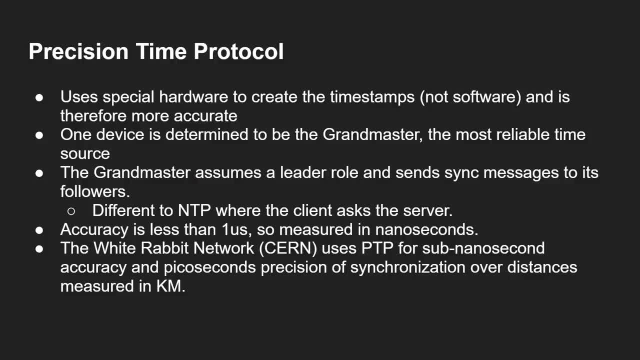 a time synchronization called the precision time protocol, PTP. Now it uses special hardware to create timestamps, So it doesn't use it through the software. Actually does it at the kind of at the network level down by the network card, And it's able to get a much more accurate timing of. 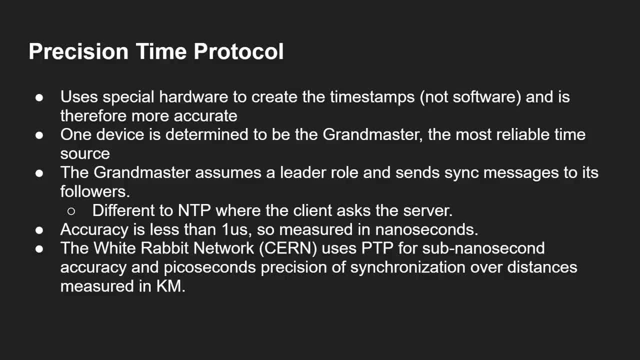 how these packets fly about on the on the network And what happens in PTP. it's a bit different to PTP. There's one node which is designated to be the grand master in any particular network setup And the ground master assumes a leader role and it sends out synchronization messages to its 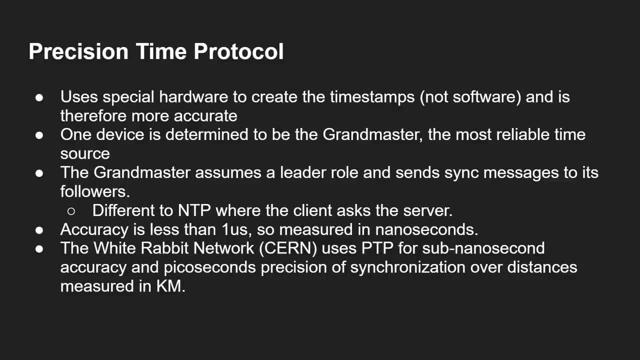 followers. So rather than the NTP client asking for the time with PTP, the grand master sends out the time. There are still some other messages that go back and forth trying to measure delay, and we'll talk about that in a minute. Now, accuracy with PTP is less than one microsecond. 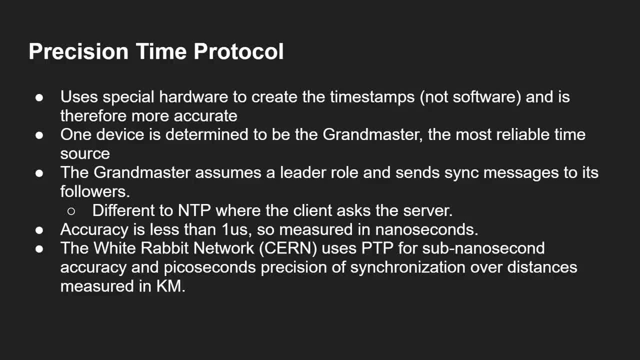 So therefore it's measured in nanoseconds. Now the white rabbit network by CERN uses PTP for sub nanosecond accuracy and picosecond precision of synchronization over distances that you measure in kilometers. So that's a really, really precise use of this technology. 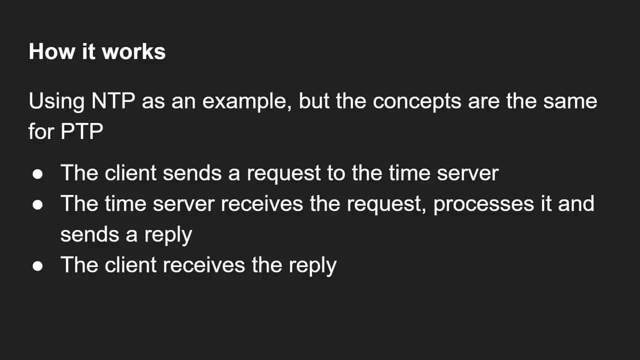 So how does it work? Well, we're going to use NTP as an example, but the concepts about delays and things we'll talk about in a minute are the same for PTP, But we'll just use NTP. So a client sends a request to the time server, The time server. 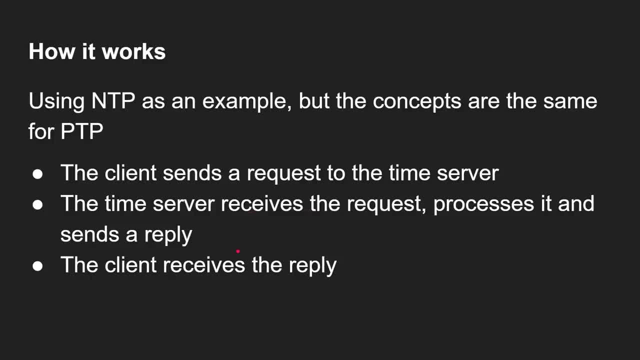 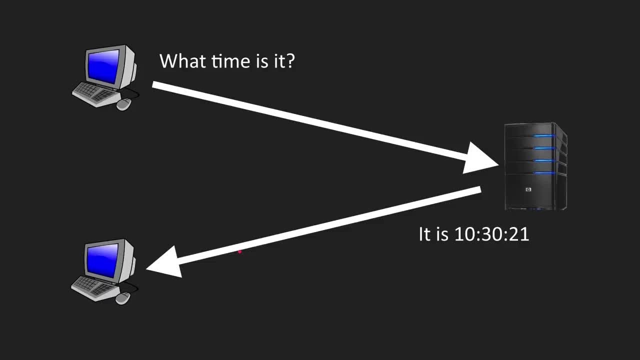 receives the request, processes it and sends back a reply. and then the client receives the reply. Basically, what time is it? It's 10, 30 and 21 seconds, and that's basically what happens. So the client asks for the time and the server gives it back the correct time. 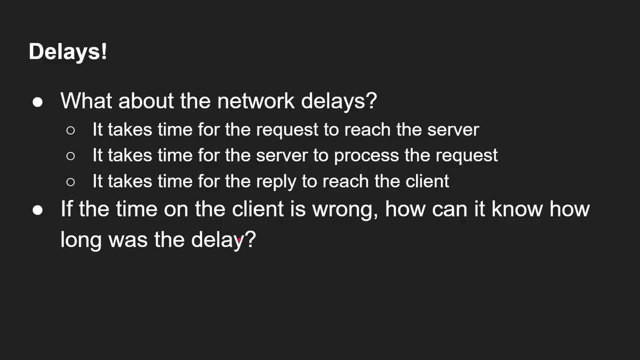 But, But What about the network delays? It takes time for the request to reach the server, particularly if you're doing it over the internet. It's going to go down through your local network, over your wi-fi, even out through the modem or the router that you've got from your network. 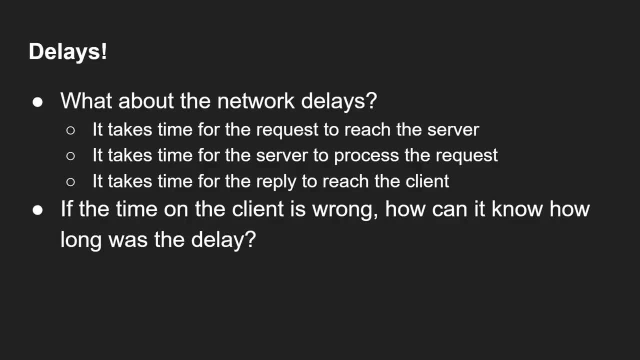 provider That goes out onto the internet might go across a couple of countries. it might hit the primary time server and then it has to process that and it's getting in lots of other requests as well. Your request gets processed and then it has to send it back. It goes over a couple of 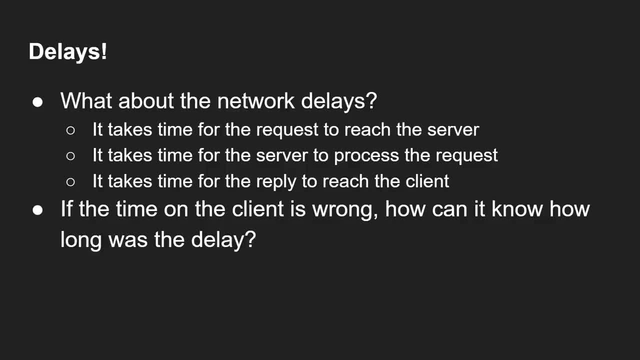 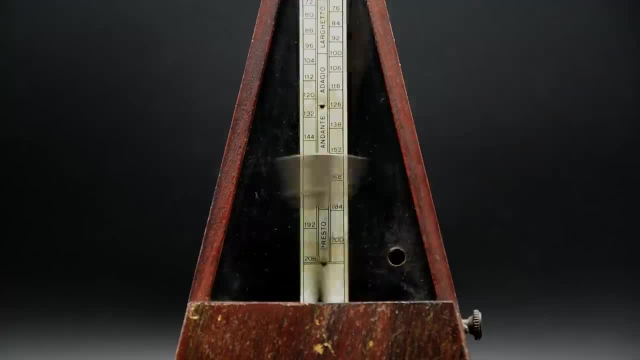 countries goes through into your local internet provider, finally comes all the way over your wi-fi to your smartphone or to your laptop and it can say: oh great, I know what the time is now And also what happens if the time on your client is wrong. So you know, it's a few minutes out, so 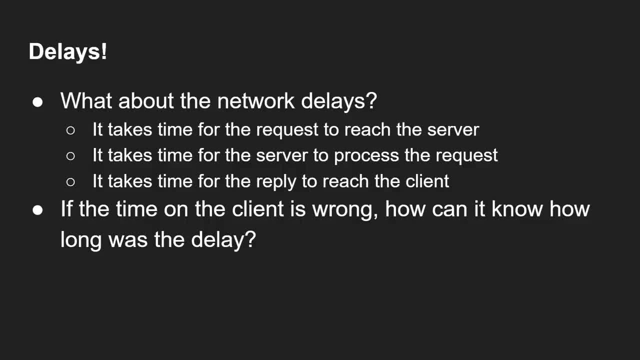 the time it gets back and the time that it's sent. they're different. So how can it know how long that took if it's trying to calculate the delay? Well, these are all very good questions and thankfully there is some very good answers. Okay, so the time that the client 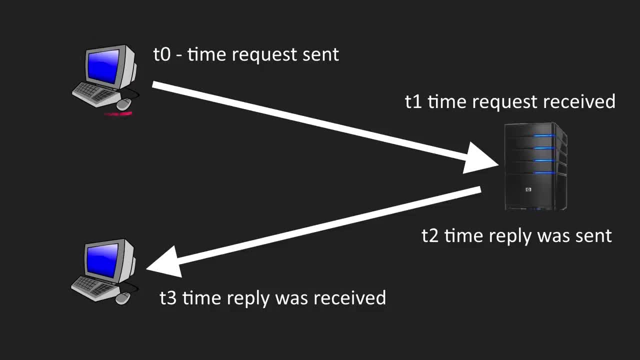 sends its request, we'll call t0.. That's according to the time that the client understands. Now it could be the wrong time, but the time it knows is the correct time. It sends the request by time that then gets to the server, It's noted down as t1. the time the 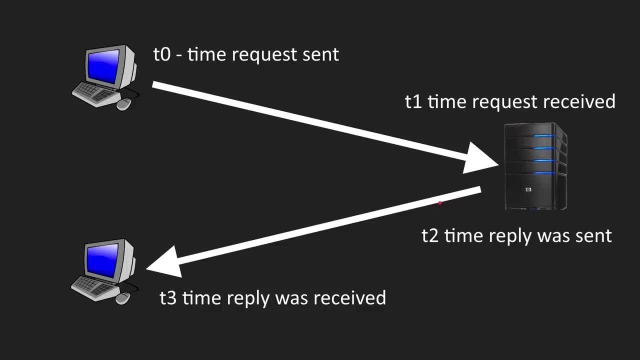 request was received. The server then processes it. It then sends back its reply. The time it sends back its reply is known as t2, which is probably the time it's also sending back, And then, finally, when it received again at the other end, that's t3, the time the reply was received. 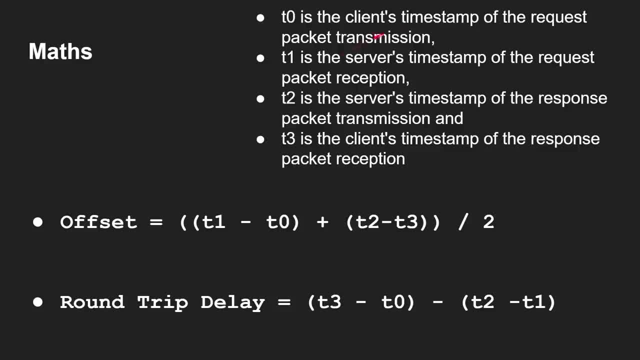 So, as we said, t1 is the time it was sent t1. received t2, the reply is sent t3.. Now here are the maths. The offset, okay, is t1 minus t0, so that's this one, the time the timestamp was received minus. 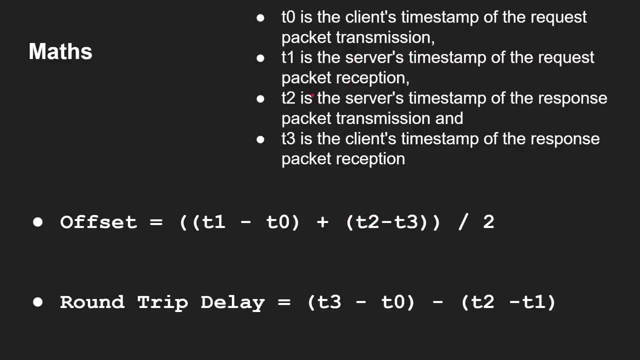 when it was sent, plus t2, minus t3, all divided by 2.. And if you, if it's the other way around, that one time is ahead of the other, you get minus numbers. you just take the absolute value And you work out the round trip delay: t3 minus t0. so t3 minus t0, t2 minus t1. And that will give you 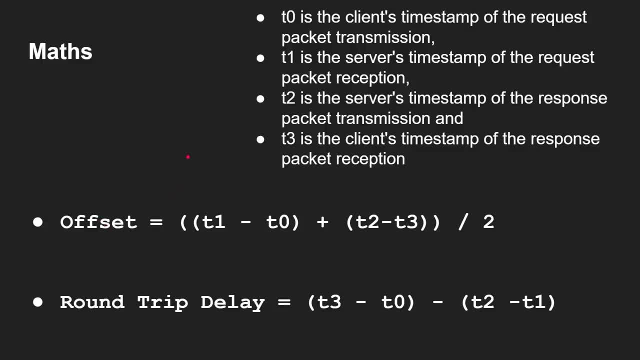 these two numbers offset and round trip delay. Well, that's all very well, just looking at the, the mathematic symbols here, but let's actually go through a working example and you actually see that it does actually work out really quite neatly. So here's our algorithm at the top, just 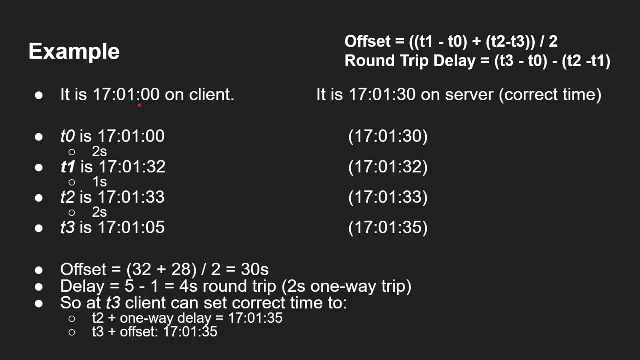 so we remember those maths. Now let's say it's 1701 exactly on the client, but that's time is wrong. the actual time is 1701 and 30 seconds, so it's 30 seconds out And on the server- our primary time server- that's the correct time. So t0 is at 1701, the wrong time, and it gets sent. 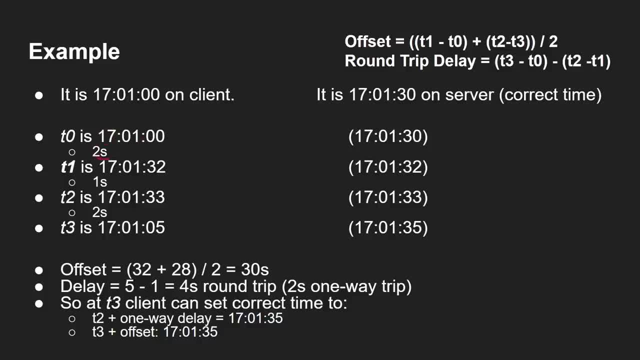 through to the server. Now, let's say it takes two seconds to get to the server. we're just using big, nice round numbers here. So t1 is 1701 and 32.. Notice, now we've gone from 00 to 32.. Why? Because 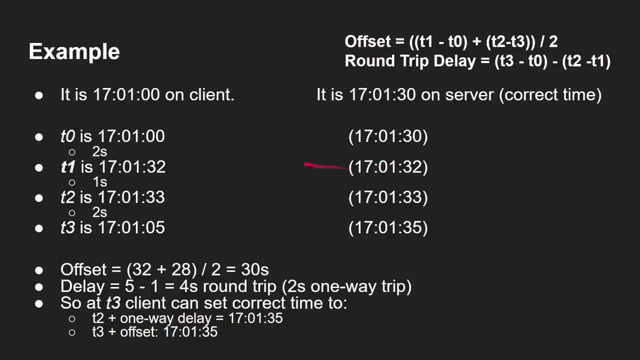 of course is 1701 and 32 because it's 30 seconds wrong. So t1 is 1701 32.. It takes a second, let's say, to process that request and then a reply is sent at 1701 33.. So 30 seconds different from the client. 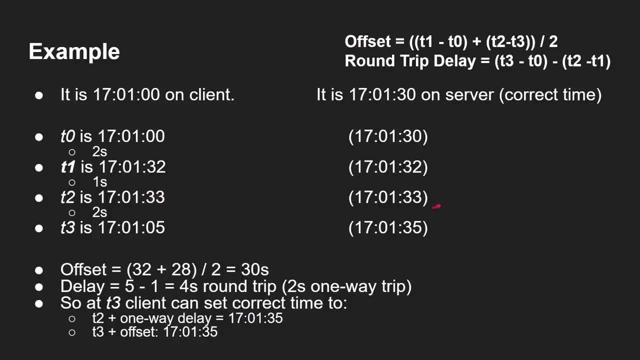 and now three seconds have gone past. So here's our real time: 17133.. And then, finally, that goes all the way over the internet and it gets to our client t3, when it's 1701, 05. now it's not 35. 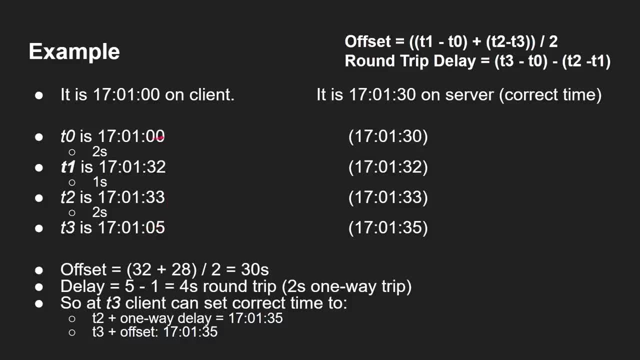 because it's got the wrong time, of course. So it's five seconds. so, from when it sent off the request, when it got a reply, let's say it took five seconds and it's got back a reply saying the time is 1701, 33.. Okay, so it knows its time is wrong, but it actually that's not the time, because at the 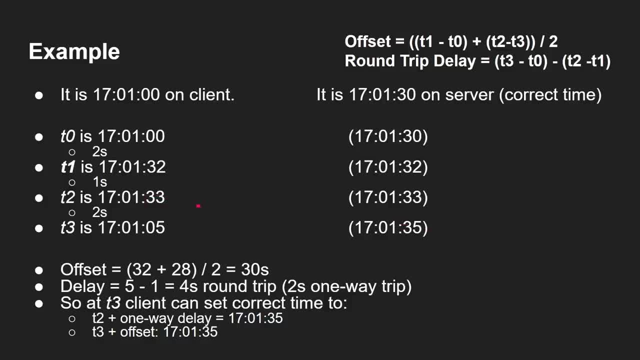 moment when it gets it's actually 1735, so it would be a two second wrong, even if it fixed the 30 second delay. it was to be wrong, But if we do the maths as we looked at, so 32. so what's that? t1 minus. 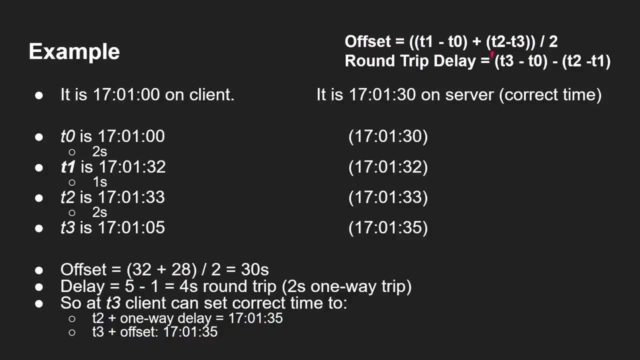 that's what we've got in there, plus 28. what's that? t2 minus t3, t2 minus 3- t3 is 28 seconds. okay, divided by 2 is equal to 30 seconds, so it's a 30 second difference between the clock on the client. 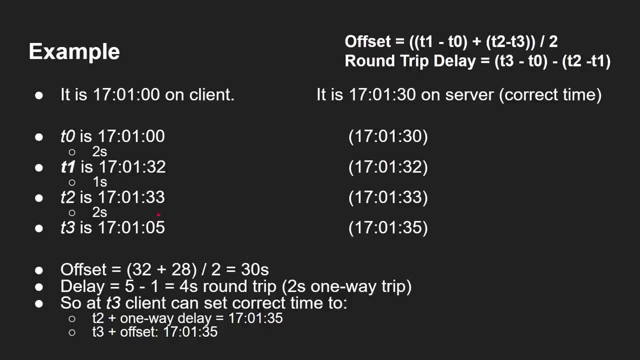 on the server. yes, that's correct, we know that. brilliant. what about the delay? well, the delay was t3 minus t0, so 05 minus that's 5 seconds minus t2. minus t1 is one second, so that's four seconds for there and back, which is two seconds for the round for a one part of the trip. so at t3 here, when the 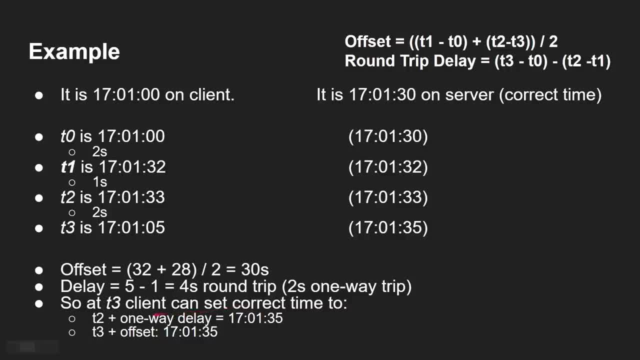 the client receives the reply, it can set the correct time to whatever was t2 plus the one way delay, which is two seconds. so it sets it to 17135, which is correct hooray, or it could take its own time. t3, 1701.05 plus that 30 seconds that we calculated, so it becomes 2101.35 and that's it. 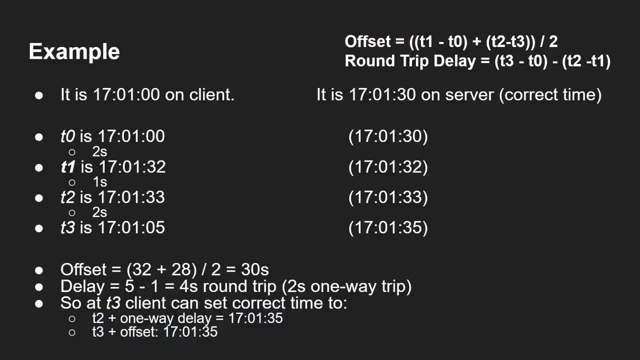 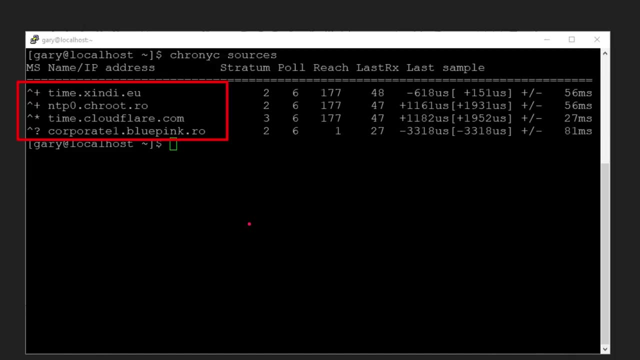 so there you can see a simple example. by the fact that the client and the server are both able to put in these protocols their timestamps, then actually we're able to work out a fairly accurate time for the client. and here's an example on a linux machine actually showing you. 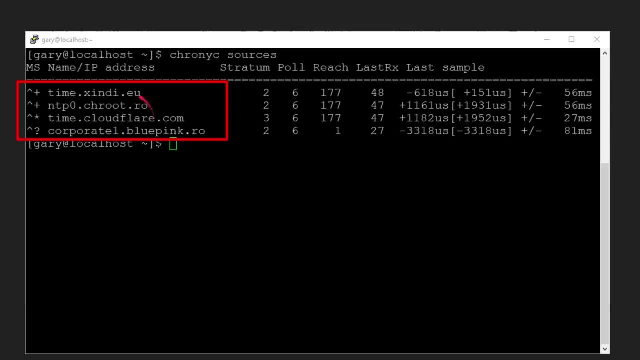 it synchronizing with some primary time servers, so you can see some here, europe and internationally, and those are the name, the domain names, of the devices that it's actually syncing to. as you can see, some of them are stratum two. there's one there, that's a stratum three.